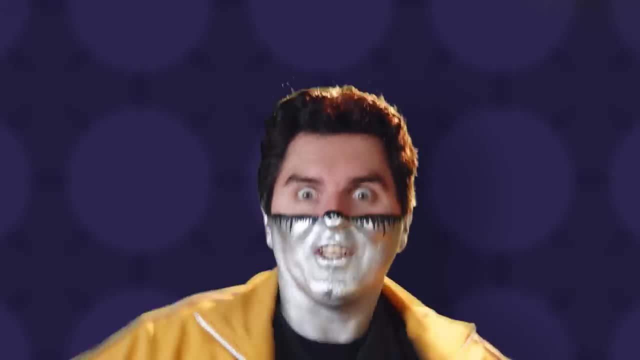 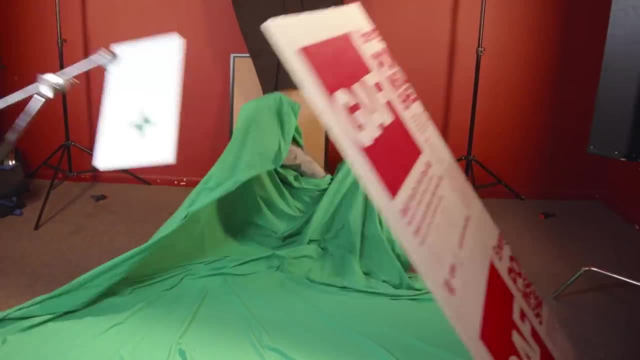 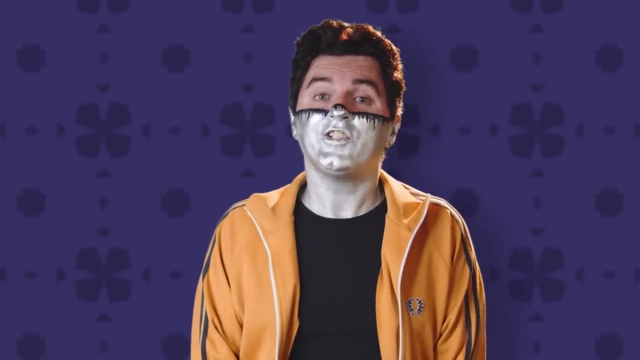 lightweight and extremely coordinated, like Ariel and me. Watch this. Okay, here we go. Oh god, I broke every bone in my body. But for the rest of you indoor types, I'm afraid the only way to meet this challenge is with the help of special effect digital visual effects graphics. Check out this guy. 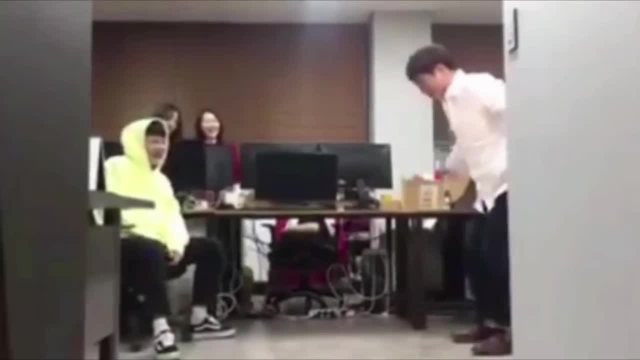 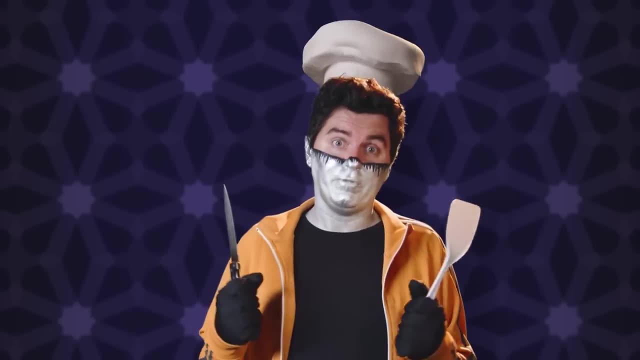 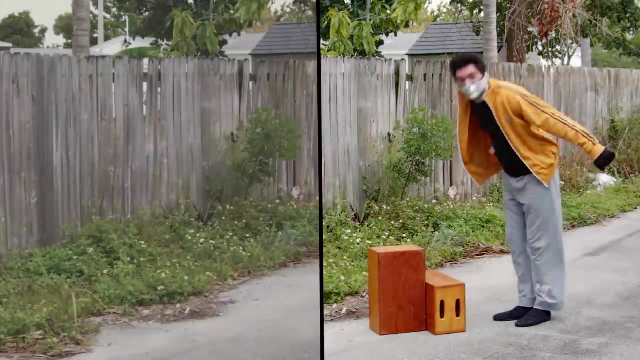 At first he really struggles, But then suddenly a double invisible step. How Well, we've cooked this recipe many times before. Shoot your scene with a static camera, Capture a blank background plate, Step on a real box. Then use some manual masking to replace the box with the empty. 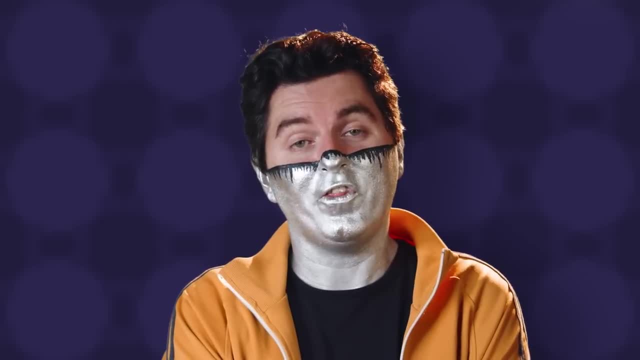 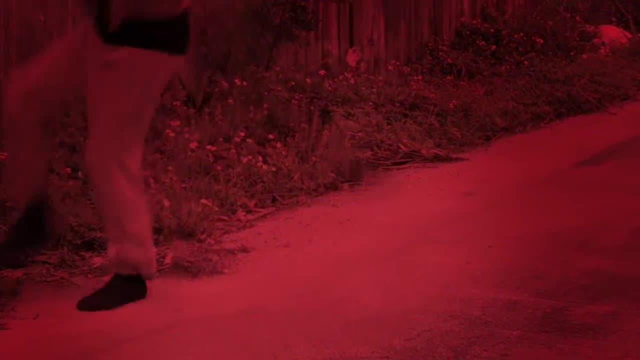 background And add some camera shake to the whole thing. Simple in theory, but if you try it, watch out for potential problems. The slightest shift of the camera can ruin the entire shot. Changes in the background make it difficult to patch And hard shadows falling where they're. 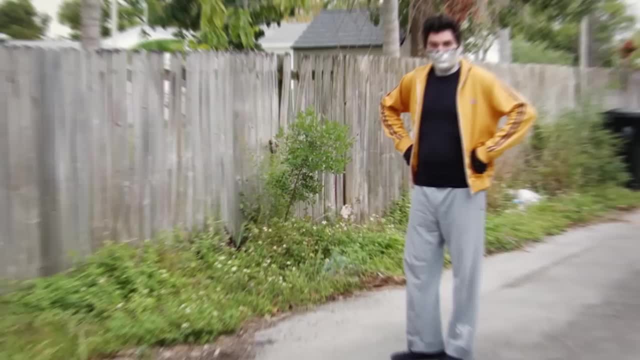 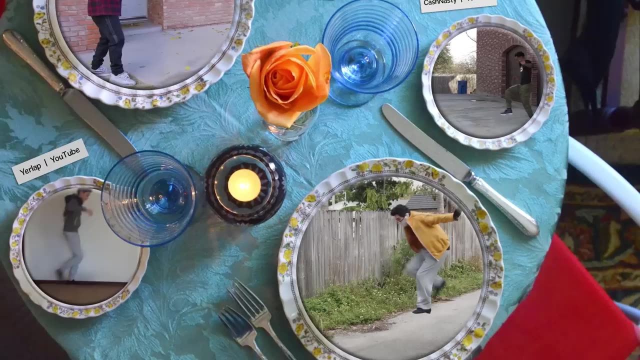 not supposed to will cause all sorts of headaches. So film on a tripod under soft lighting and you'll end up with a nice, safe fake video that looks as good and bland as a million other trick videos out there. Only that doesn't feel like much of a. 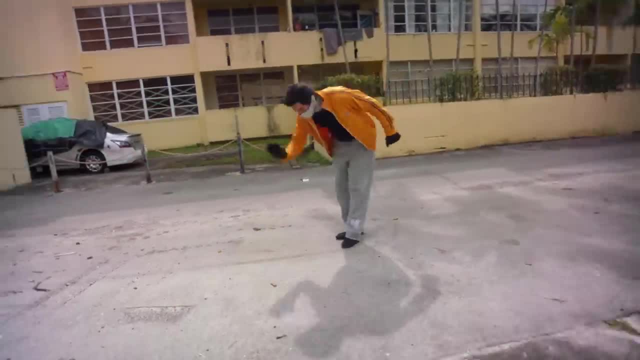 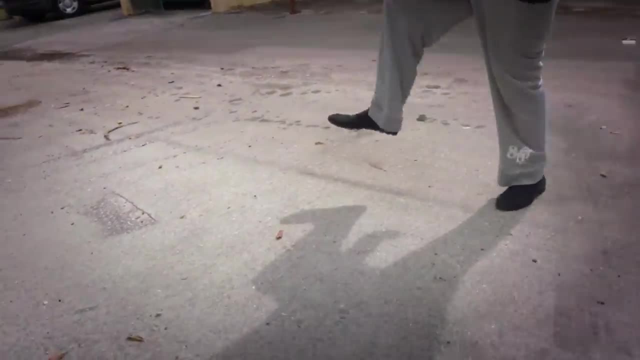 challenge. So how about this? My totally fake invisible box video breaks all those rules. The camera is handheld and moving. A clear shadow shows my foot not touching anything And this alternate angle shows I wasn't suspended from above. Can you tell how I did it? 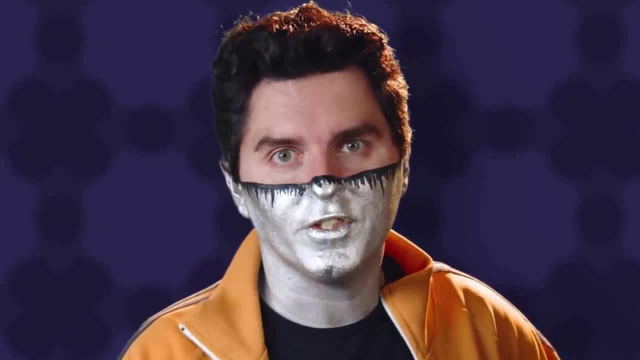 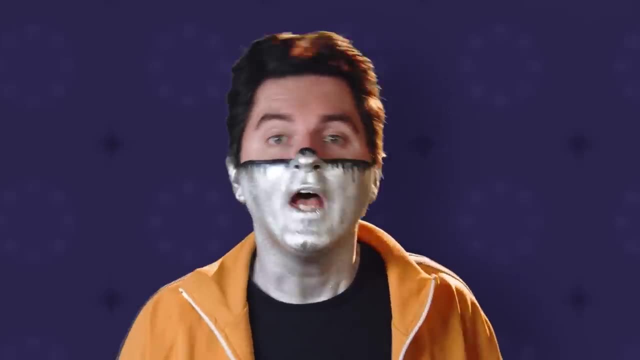 I'll reveal the answer on this day, in 10 years. So stay subscribed and click that bell. I can't wait that long. I'll just tell you, Okay, After finding just the right location on the mean streets of Los Cajas. 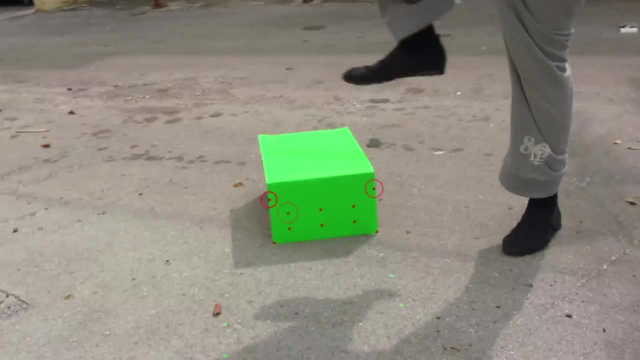 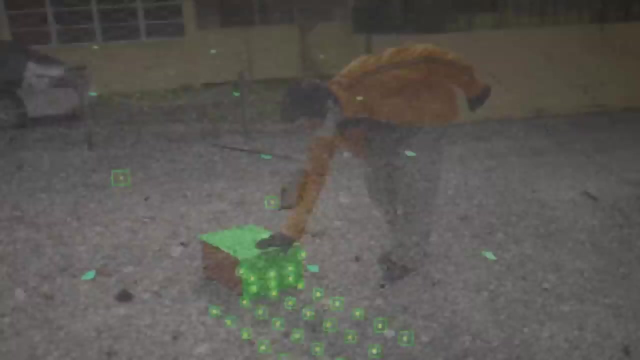 I filmed the shot with a real box dotted with tracking markers. I also put a dense grid of markers on the ground in front of the box. Knowing the exact distance between all these markers helped me extract a camera, solve and recreate the move in 3D. 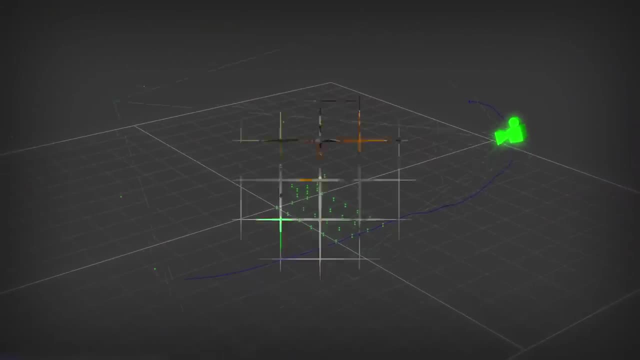 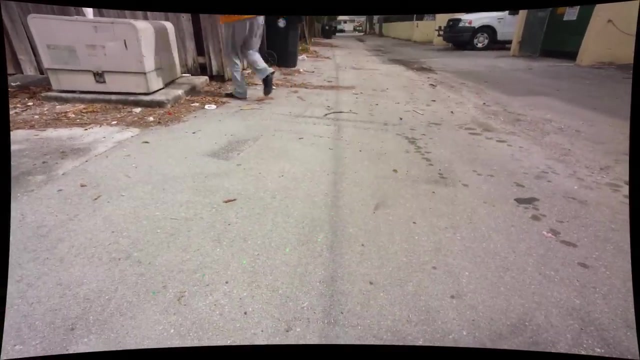 much more precisely than could be done with auto tracking. Armed with this 3D animated recreation, I was able to freeze one frame of the pavement without the box, which I made sure to capture right after filming the move and project it back onto the virtual.